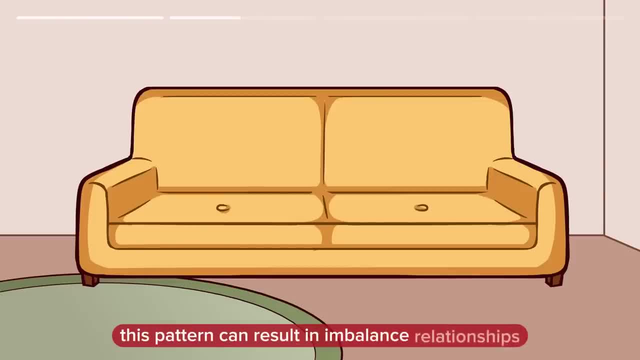 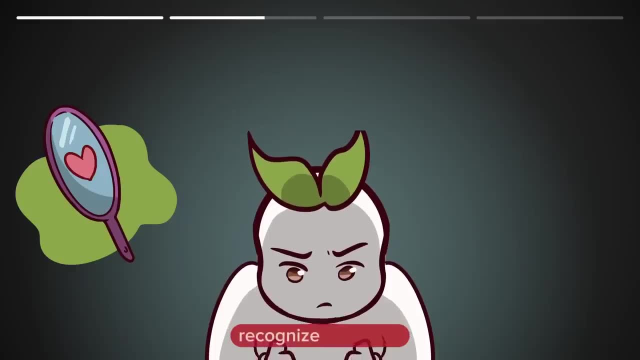 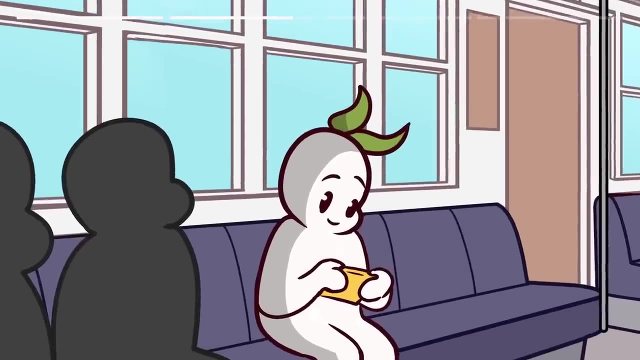 partners. This pattern can result in imbalanced relationships where emotional investment is lopsided. Understanding this empowers us to cultivate self-worth, recognize our value and seek relationships where we're genuine. So if you're finding this insightful, remember to engage with it by liking, commenting. 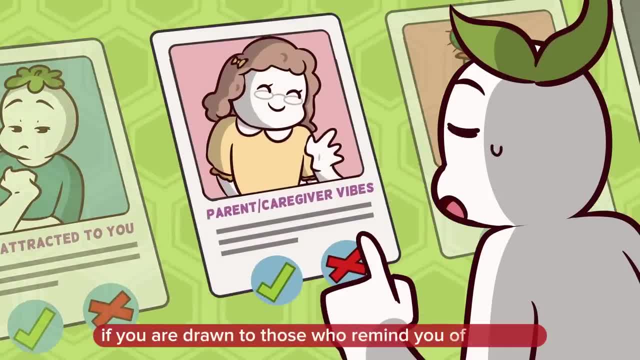 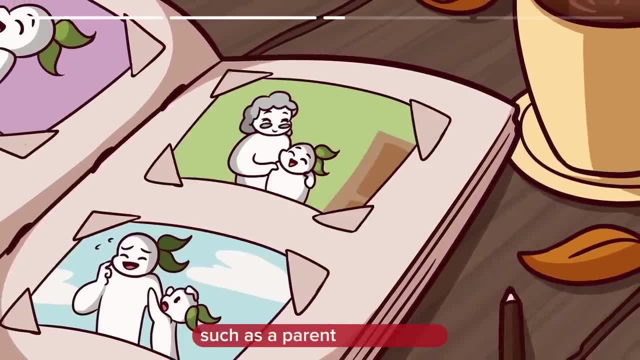 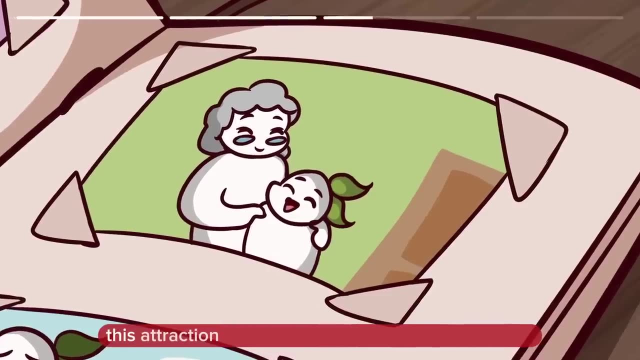 and subscribing to our channel if you're drawn to those who remind you of a parent or caregiver. Attraction to individuals who resemble significant figures from our past, such as a parent or caregiver, is a common phenomenon known as imprint attraction, explains Dr Claire Jack. This attraction can be driven by unconscious desires to recreate. 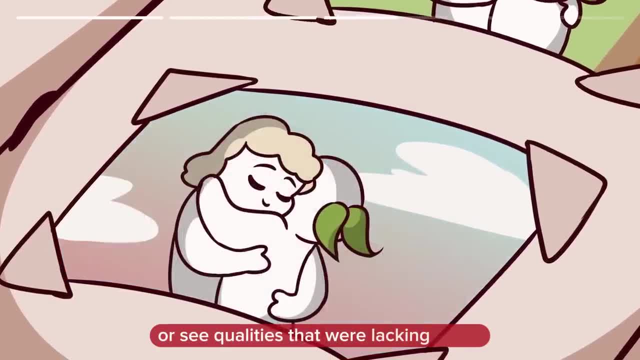 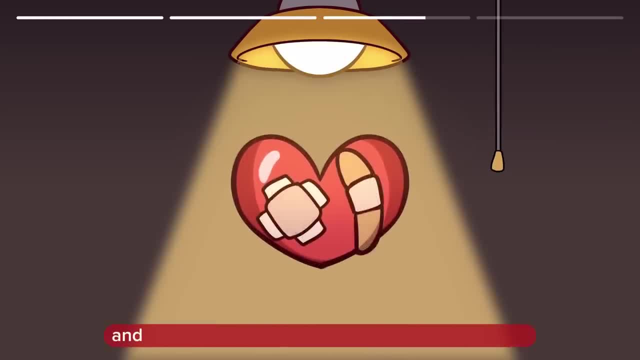 familiar dynamics or seek qualities that are not necessarily the same as those of a parent. It can be driven by the lack of relationships that were lacking in our earlier relationships. Understanding this pattern can help shed light on unmet emotional needs and provide an opportunity for healing and growth. By recognizing the influence of past experiences, you can strive. 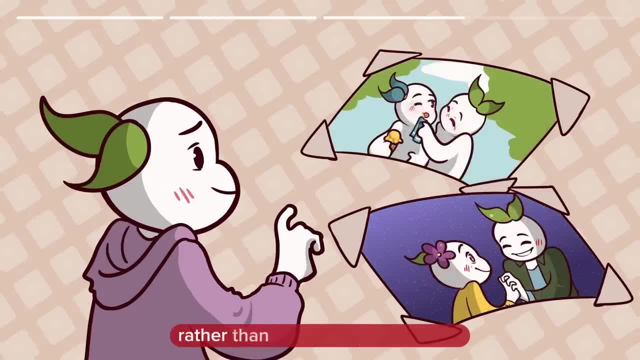 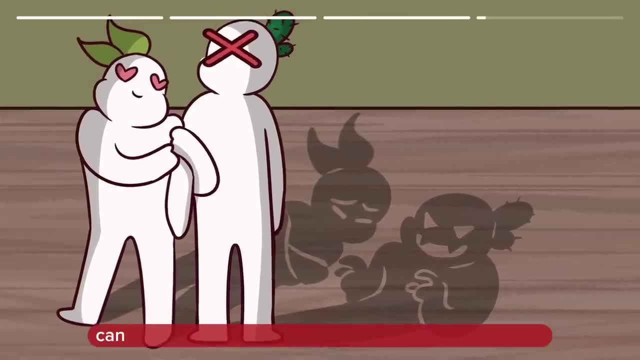 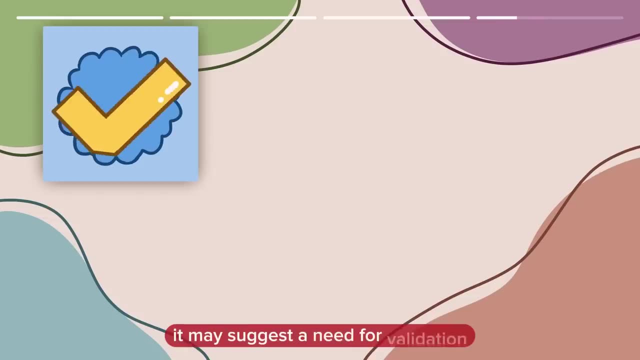 for relationships that are based on genuine connection rather than unconscious repetition, If you are attracted to toxic people. attraction to toxic individuals can be indicative of underlying issues within ourselves, says psychologist Dr Claire Jack. It may suggest a need for validation, a fear of intimacy or a pattern of seeking out familiar. 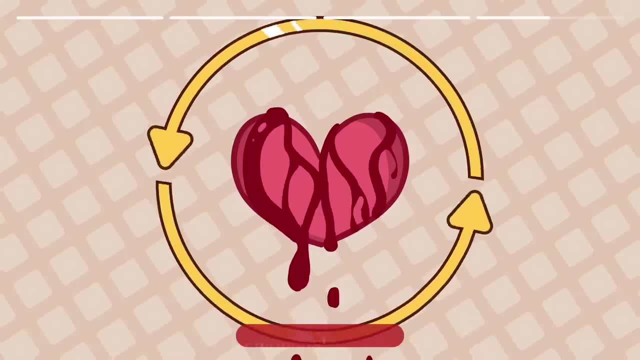 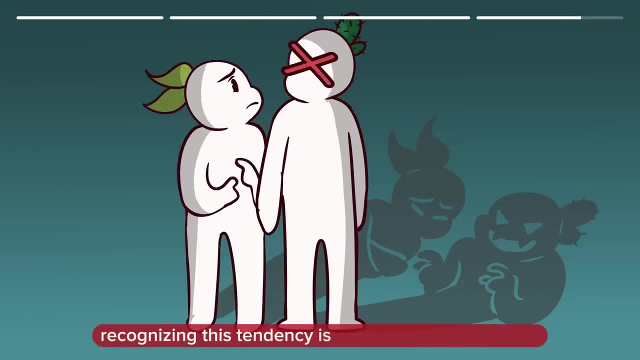 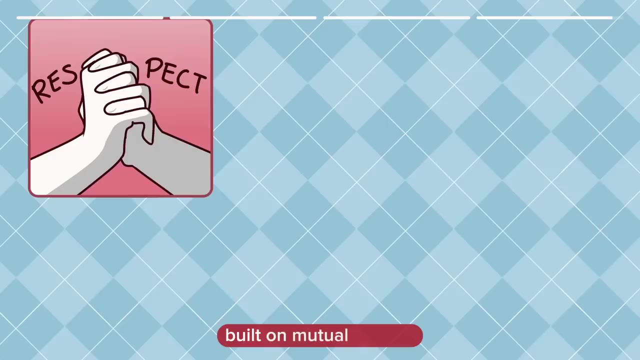 dynamics. This attraction can stem from unresolved emotional wounds, causing you to recreate unhealthy patterns from your past. Thus, recognizing this tendency is crucial for our well-being, allowing us to break free from toxic cycles and cultivate healthier connections built on mutual respect, trust and emotional support. If you're interested in learning more about the psychology, 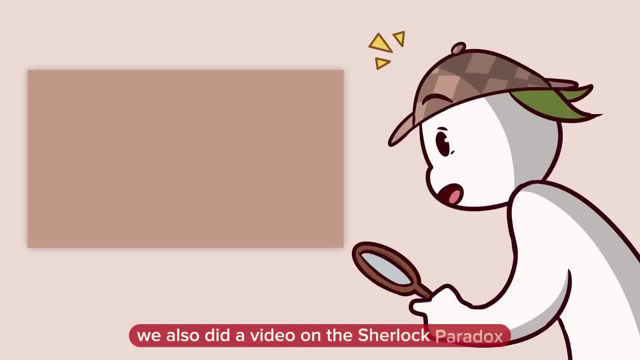 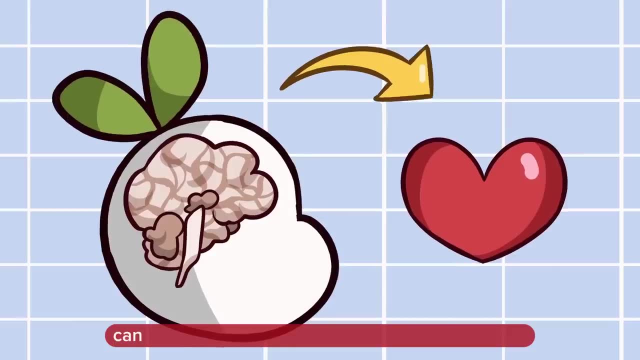 of attraction. we've got a lot more to tell you about, So if you're interested in learning more about the psychology of attraction, we also did a video on the Sherlock Paradox to attracting your crush, Because understanding the underlying many factors that underpin our attractions can help us. 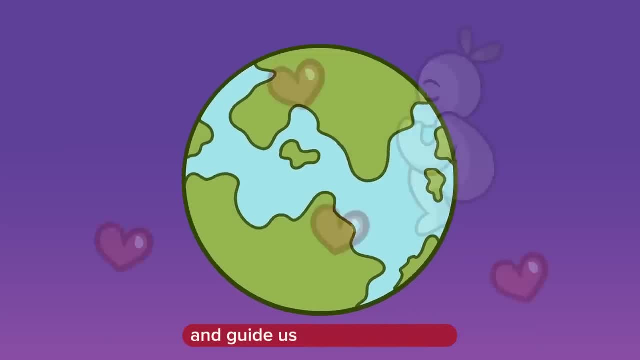 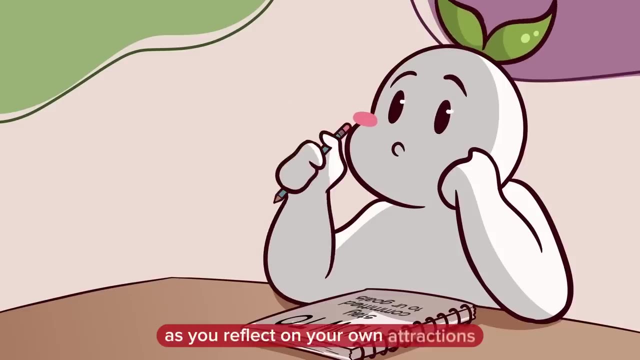 gain insight into our own personalities and guide us in forming deeper and more fulfilling connections with others. So, Psych2Goers, as you reflect on your own attractions, ask yourself: what do they say about you? How can you use this knowledge to foster healthier and more? 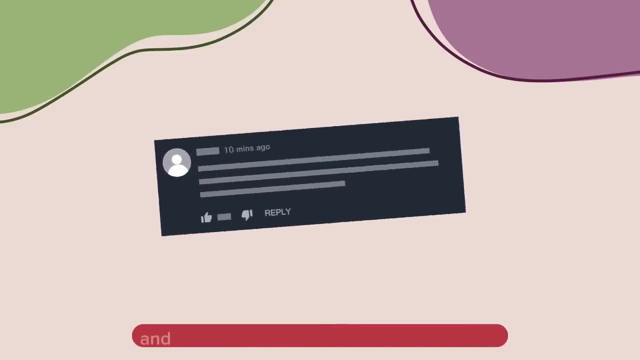 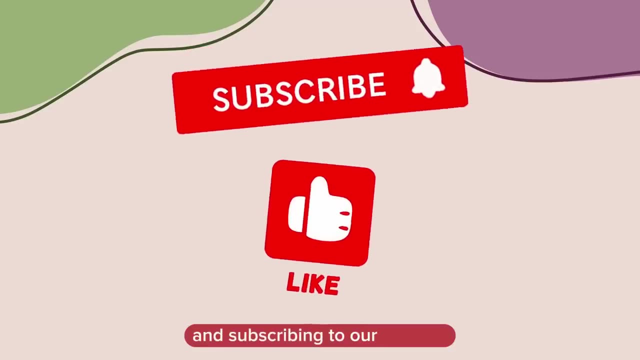 fulfilling relationships. Let us know in the comments down below, And if you found this video valuable or helpful. please support our work by hitting like on this video and subscribing to our channel.